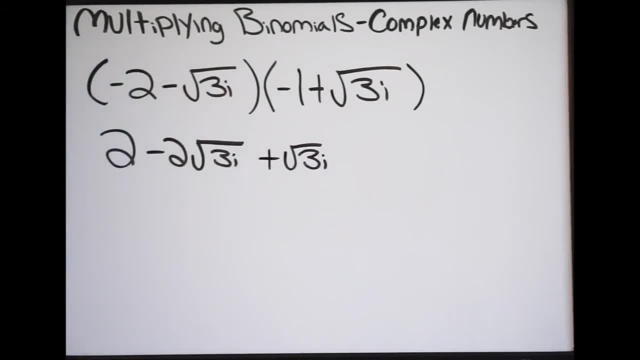 square root of 3i times square root of 3i, That's going to give me negative 3i. Okay, so now, at this point, I want to go ahead and combine my like terms, which I have here and here. So, doing this out, I'm going to get 2 minus the square root. 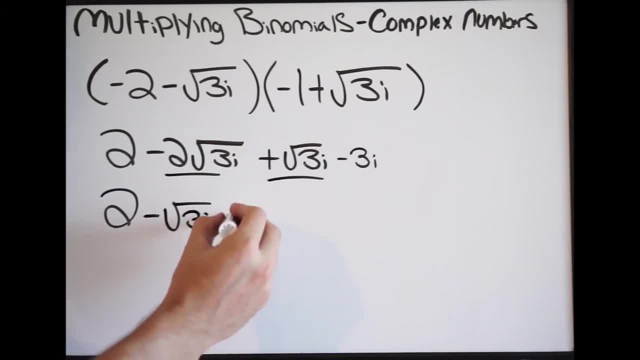 of 3i. Okay, minus 3i. Okay, and that's actually going to be our final answer. We can't combine any like terms. This right here is going to be our final answer, Okay, so let's try another. 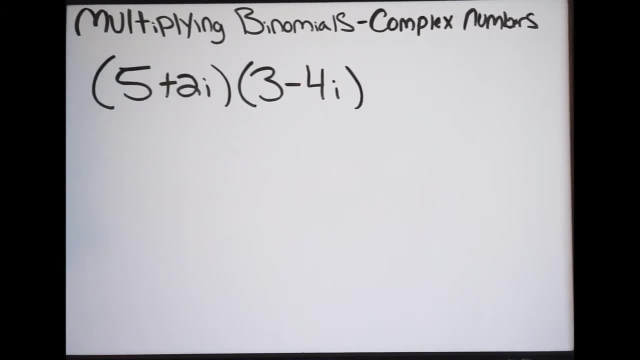 example. Okay, so here's our next example. Again, we have two binomials that are complex numbers and we're asked to multiply them. So again, we're going to use FOIL. So doing first, we're going to. 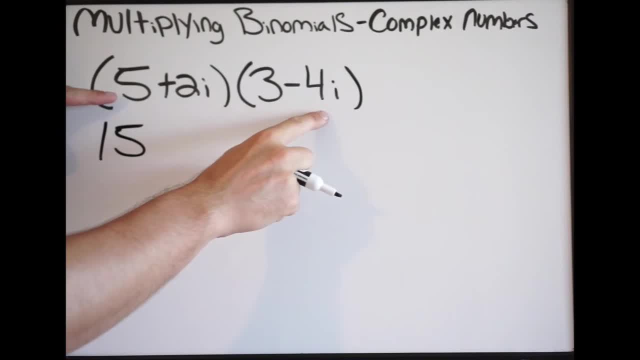 get 15.. Okay, doing outside, we're going to get negative 20i, Inside, we're going to get positive 6i And then, doing last, we get negative 8i squared. So at this point we want to go ahead. 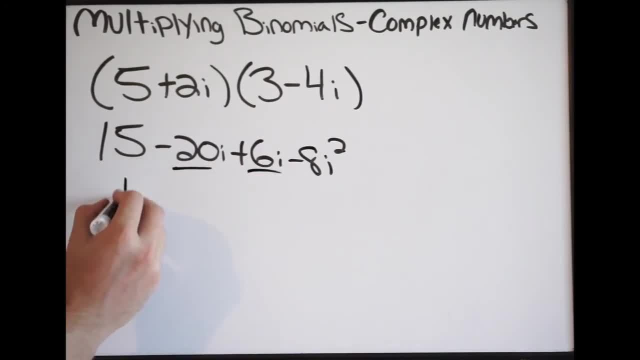 and combine like terms. We can go ahead and underline them Here and here, So we're going to get 15.. So negative 20i plus 6i, that's going to give us negative 14i. We can go ahead and cancel those out, so we know we're done. And then we get negative. 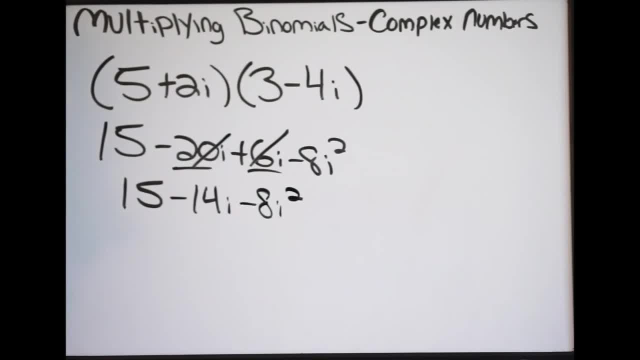 8i squared. Now remember what i is: i equals the square root of negative 1.. So if we simply square both sides, we know that i squared is equal to negative 1.. So wherever I see an i squared, I can actually replace that with a negative 1.. 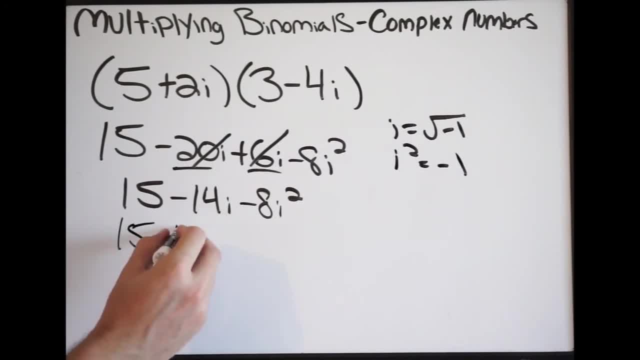 So, for example, I have 15 minus 14i minus 8 times a negative 1.. This is now going to become positive 8, right, So we get 15 plus 8.. Okay, we know that that's going to give us 23.. So we get. 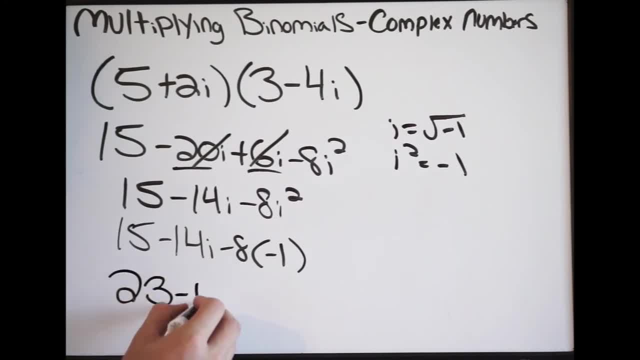 23 minus 14i. And this here is going to be our final answer. Remember, when you're writing a complex number, you always want to have it in the form of a plus bi, meaning you have your real part followed by your imaginary part. Okay, so this here is our final answer. All right, and 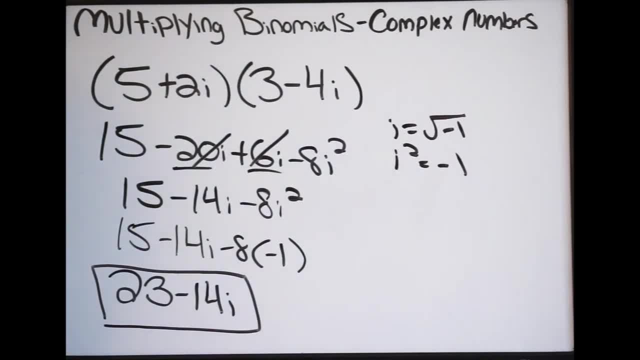 that's multiplying binomials, that are complex numbers. Okay, and that's it.